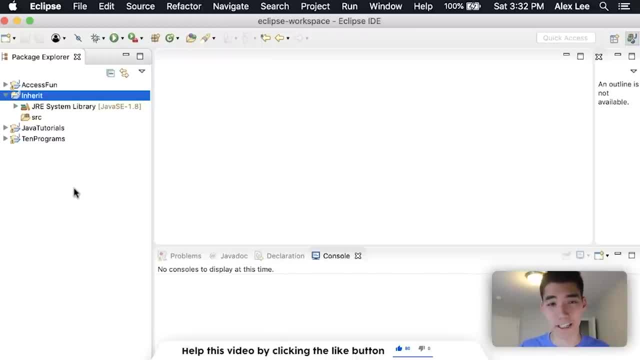 gaming mice, but we also need to write the software for each of the gaming mice. It's like cool. yeah, I'm excited, but how do we start that? I know how to make a for loop, but how's that going to help me? 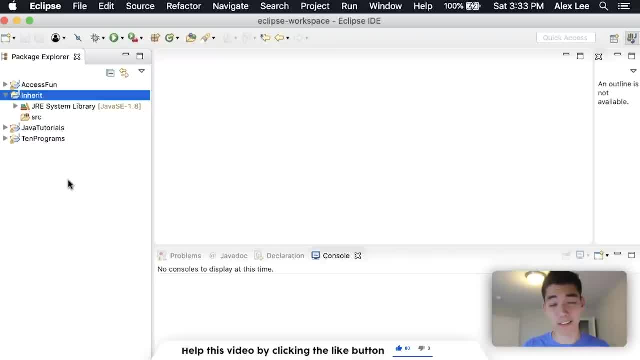 like make a mouse and program one. Java solves this problem for us through its nature of object-oriented programming. What we can do is we can create objects for different mice, and so, yeah, we'll try to do that. We'll try to create five gaming mice as objects in this project. So we'll go. 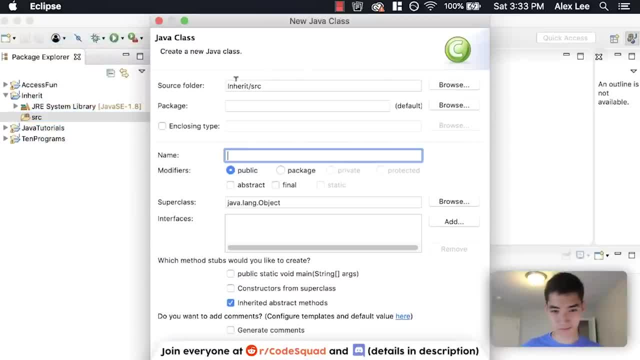 to File New Class, and in this video we're going to work on three of them, just because five is going to be too many, So we'll call it like mouse1.. finish, and it'll make two more: mouse2 and mouse3. 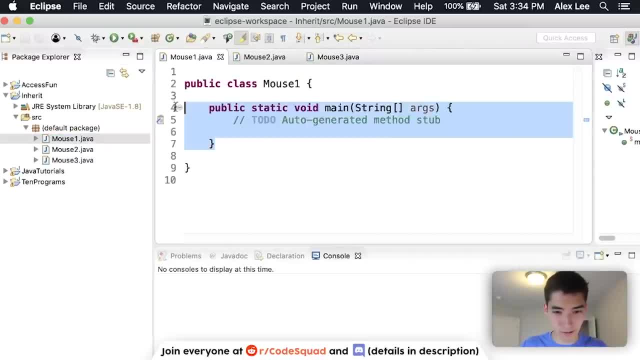 So we've got our three mouse classes here. I'm just going to remove the main method. That was an accident, so they should all be empty classes like this. And don't worry, we'll get to inheritance in a second. but 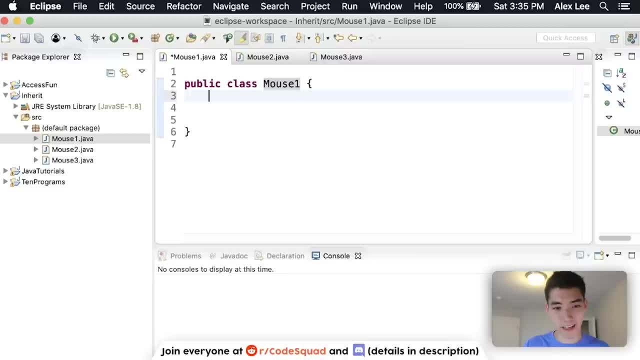 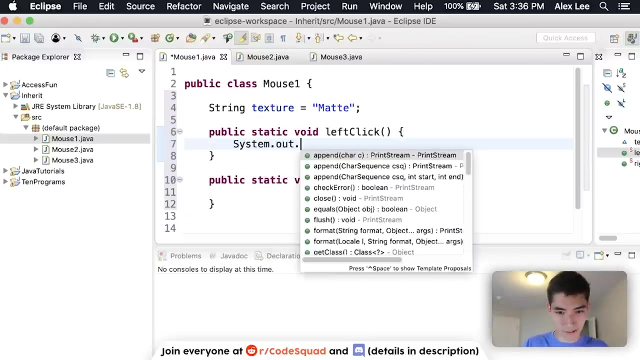 let's just start making these mouse objects and start making them pretty cool. We'll say: one mouse is like a cool matte black texture. We can set the texture equal to matte. Of course it has left and right click. so we'll make some methods like left click and right click and for simplicity's sake we'll just 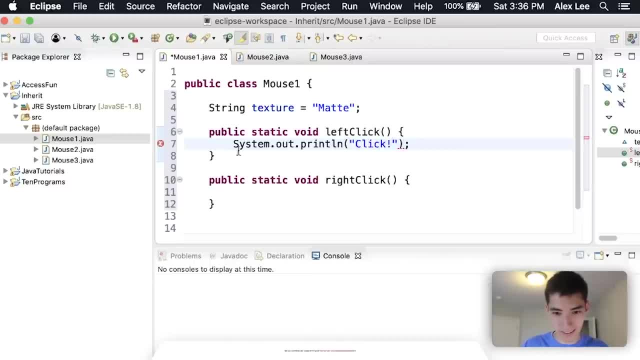 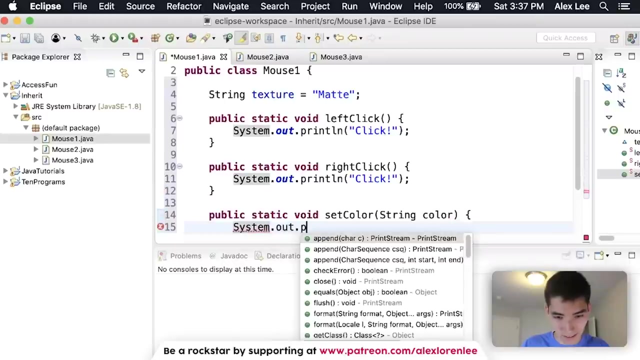 print out click like that in each of them. The mouse one also has another cool feature: it's also got some, some RGBs on it, so we can set a certain color and we can say which color, and we'll print out that it's that color. Let's go. 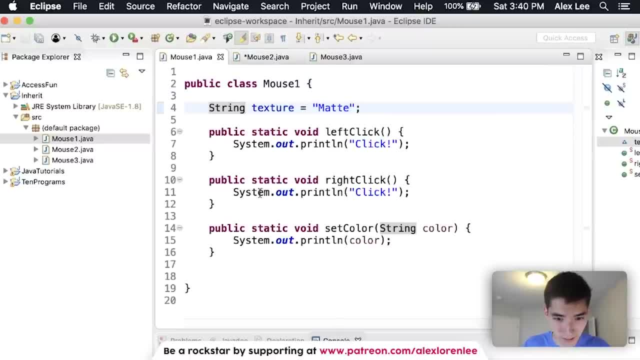 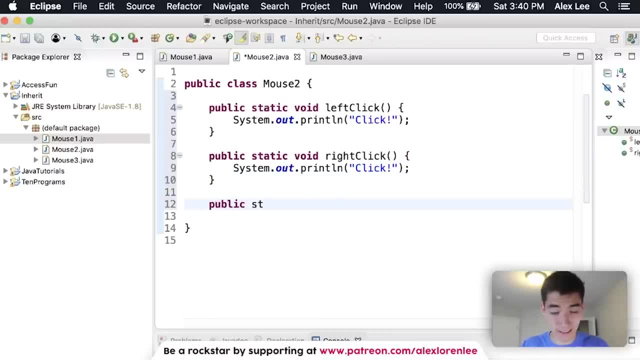 on over to mouse two. It can also do left click, right click, so I'm just going to copy these over. and let's say, it's special feature that makes it stand out is that it's Bluetooth, so we can have a method like connect, Connect. 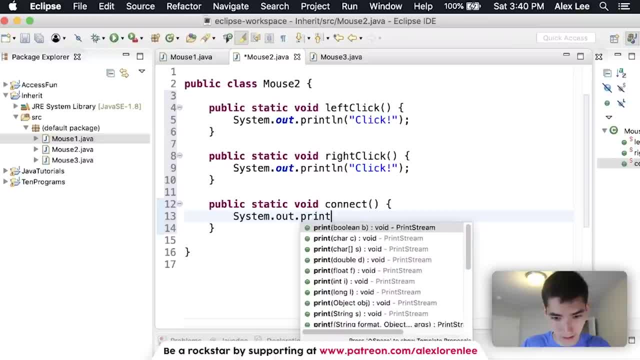 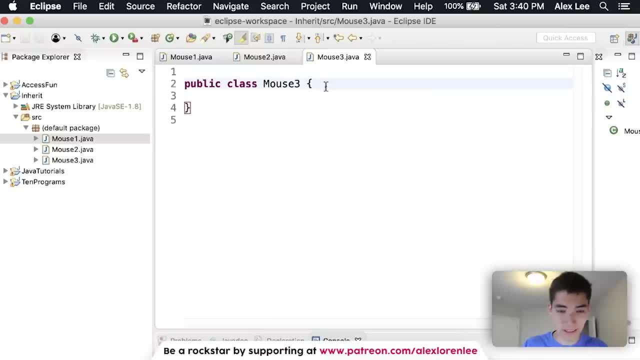 And we can connect to Bluetooth. and finally, mouse three also knows left click, right click. so we'll copy and paste that over here, but its special feature is that it's ambidextrous. so we'll actually just have that like maybe as a property here and say: boolean, ambidextrous. 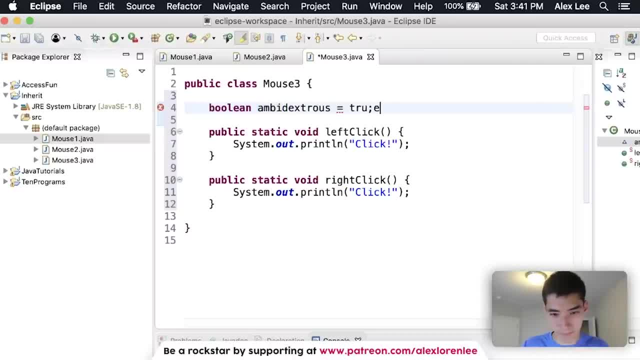 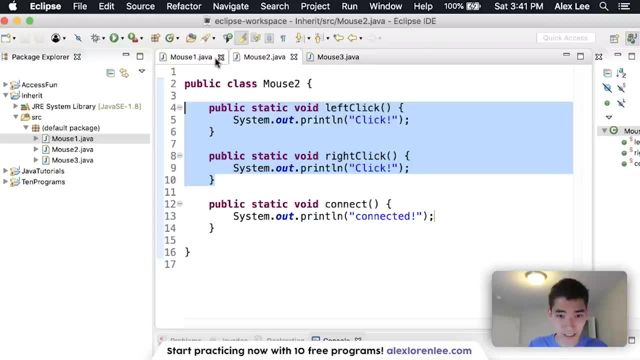 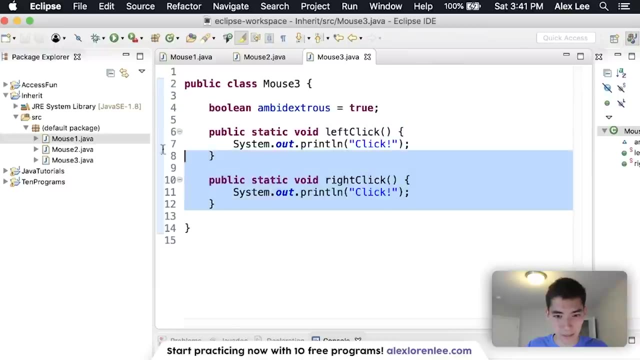 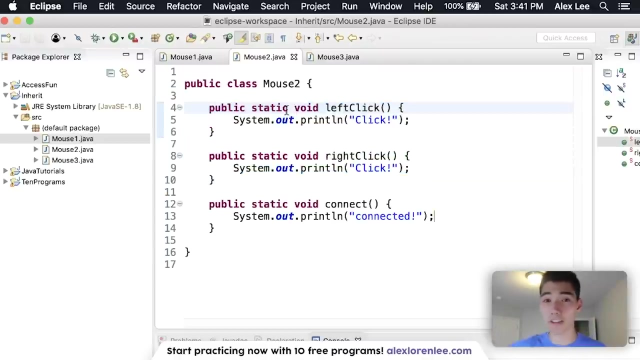 equals true, something like that. so we've got three mouses here, each slightly different. they all know how to left click, right click, and so repeating this code a lot can be pretty redundant. it just makes it difficult to keep track of. and if our company grew and we had to make a hundred different mice in a year? 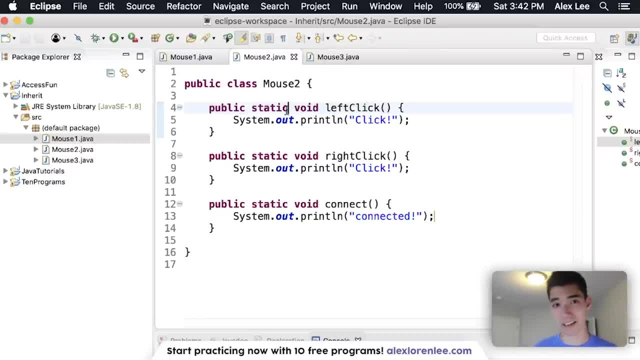 then copying and pasting this a hundred times. it's not gonna make sense to keep track of the code any easier to read. so we can make as many mice as we want that have different features by making a generic mouse that has the basics like left click and right click. so to do that, 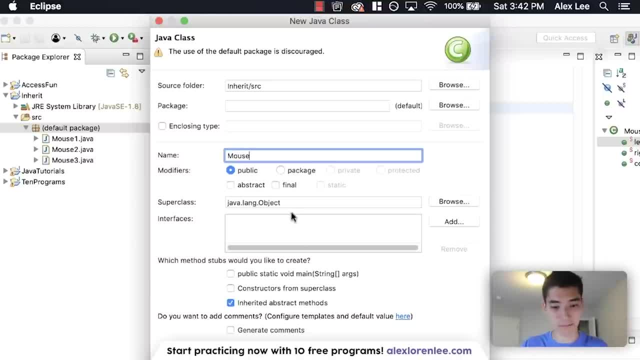 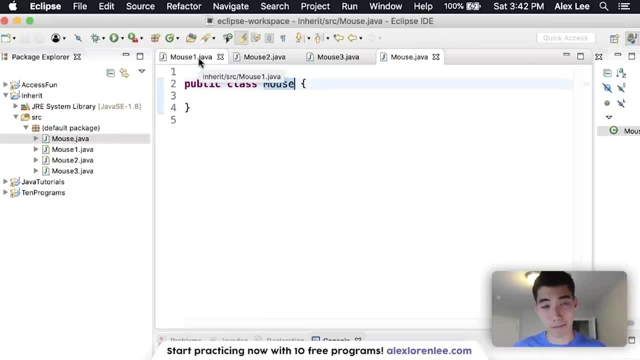 we'll just go to new class again and we'll just call this mouse and hit finish and our generic mouse is going to have everything that all of our mice is going to have, and all of our mice are going to have left click, right click, so we can just take that and put it in here. 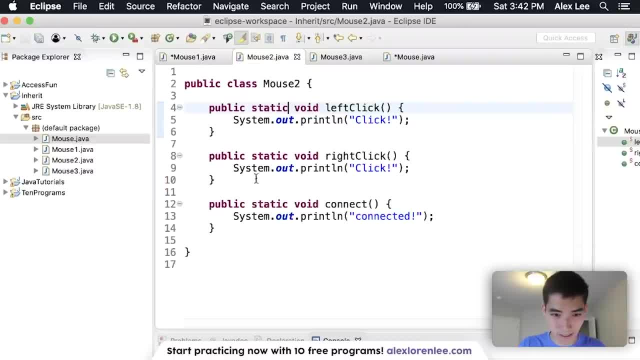 so that way it doesn't need to be in mouse1, it doesn't need to be in mouse2 and it does not need to be in mouse3. make sure all of these are saved. and let's say also: all of our mice are going to have a scroll wheel, so we can do the same thing. let's scroll up. 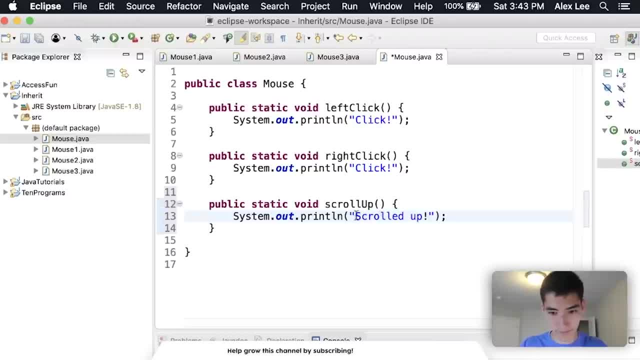 scrolled up and scroll down. in real life. these would be implemented like there'd be code in here, like if statements and for loops and parameters. but it wouldn't be as easy to show in the console here in a second when everything comes together. so now we have our generic mouse. 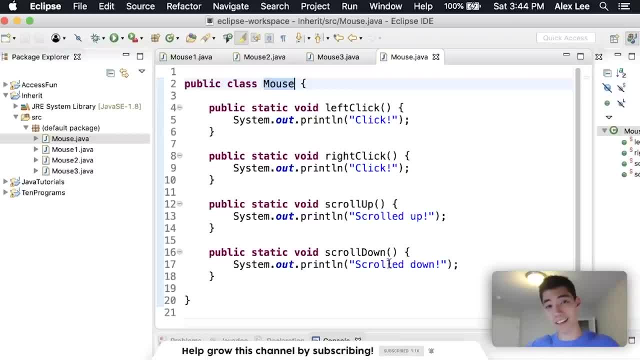 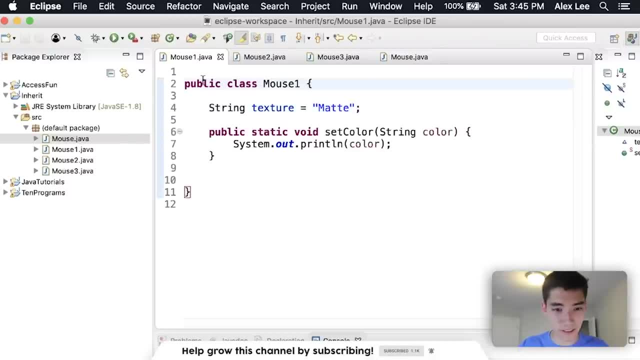 that can left click, right click, scroll up and scroll down. we can create a ton of other mice based on this and that's called inheritance. and to do inheritance is super simple. you just go up to the name of your first mouse and do extends mouse. okay, seems pretty easy. let's just do that to mouse2. 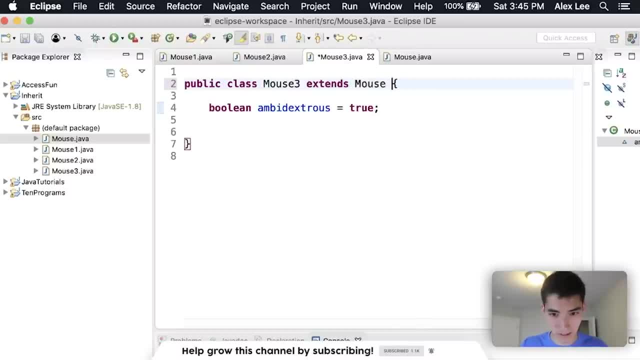 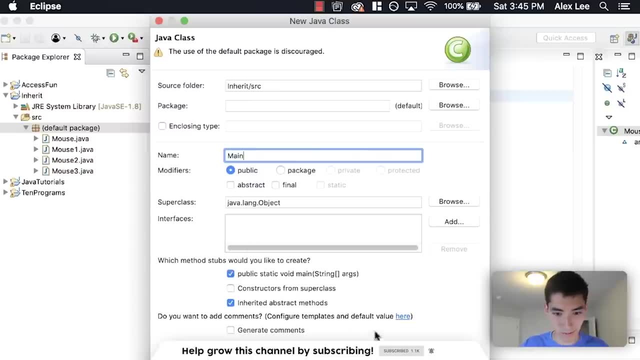 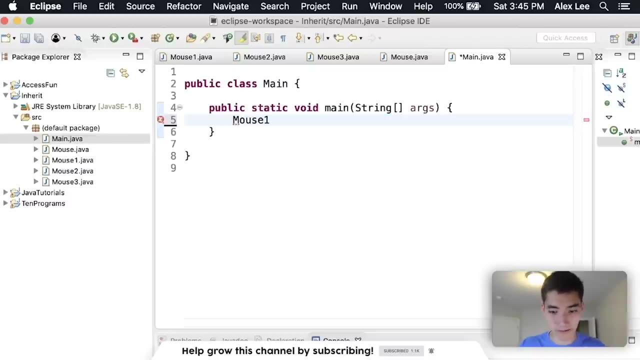 and also mouse3. now, if we created a main method here to see what's all going on here, rn1 a style and hit a public static void so we can run our code. if we create our first mouse mouse1, call it m1 equals new mouse1. 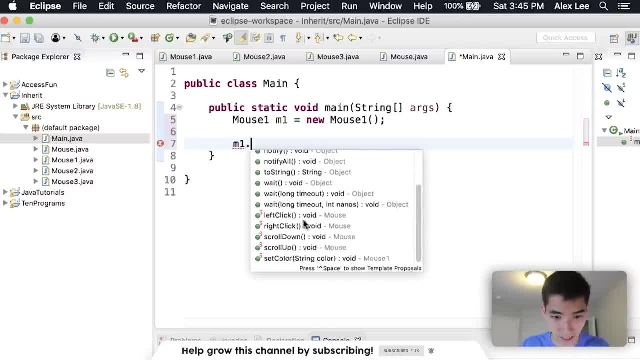 if we do m1 dot, we can see everything that that mouse one can do and we can see that it has a texture and it can also left click, right click, scroll down and scroll up, even though. But when we go to mouse1, we don't see scroll up or scroll down. 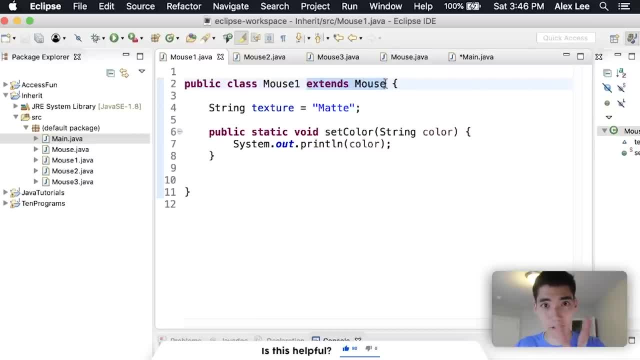 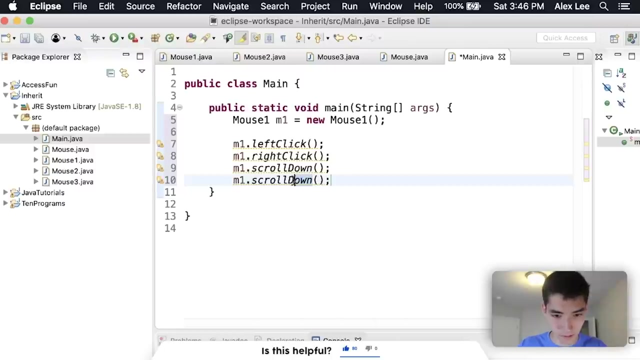 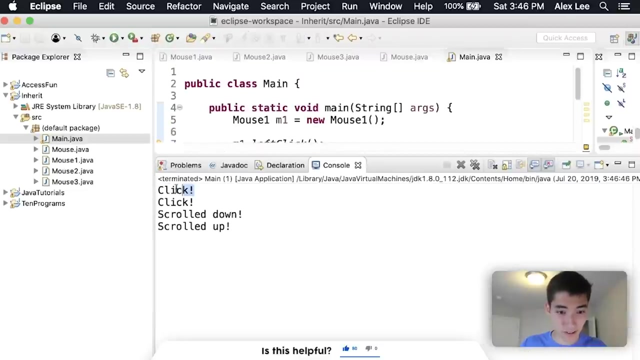 But since it extends mouse, these two keywords mean inherit. Since it inherits from the generic mouse, it knows everything already And that's why it knows left click, it knows right click and it can also scroll down and scroll up. And if we run this, we'll actually see those methods being called. 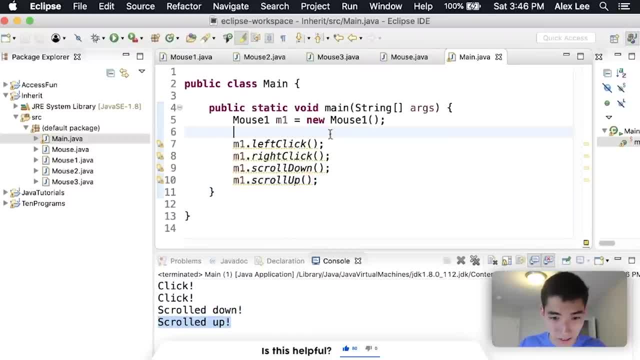 Click, click scrolls down, scrolled up, And this happens too with all of them. So if we change this to mouse2, the same exact thing would happen. Two, two, two, two And there you go. But we also have. 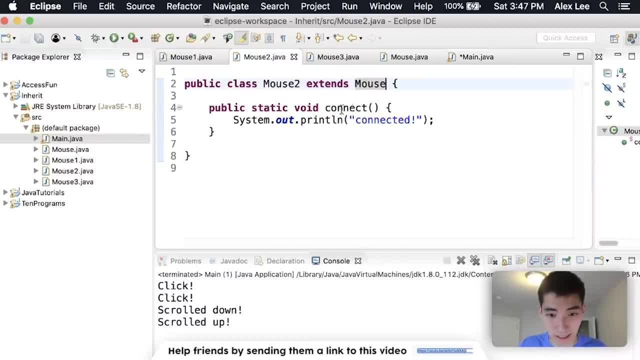 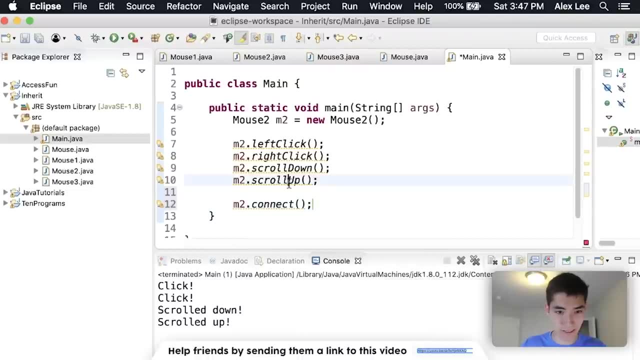 The property is specific to mouse2.. We see connect, the method connect. Since mouse2 is Bluetooth, we can do m2.connect Like that, And now we see that connected message. But we can't, for example, get a texture because there's no texture in mouse2.. 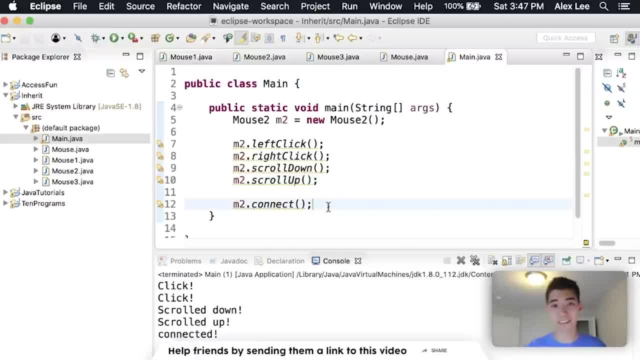 There's only a texture in mouse1.. So what this does is it lets us create a generic object and then we can create a bunch of different variations of it And keep track of it all the time. It makes it a lot simpler.